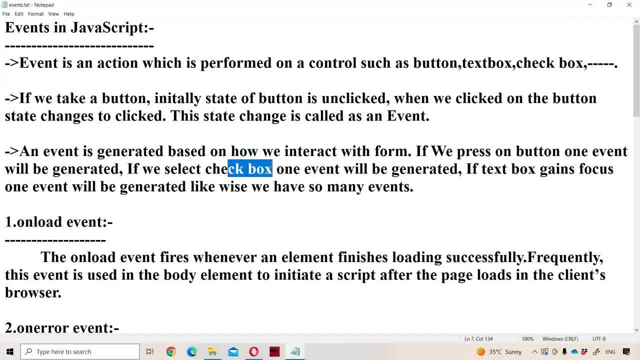 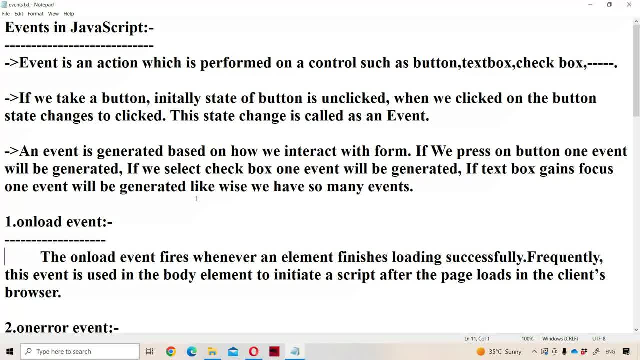 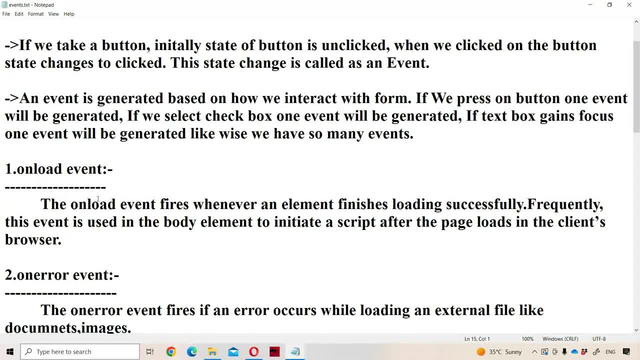 So we have several events are there In this video. mainly we are focusing on 10 important, very, very important events. The first event is onload event. Onload event finds triggered, executed whenever an element finishes its loading successfully. Secondly, frequently this event is used in the body element to initiate a script after the page loads in the client's browser. So onload event is mainly executed on body tag. So whenever a web page is loaded in the browser successfully, then onload event will be executed. 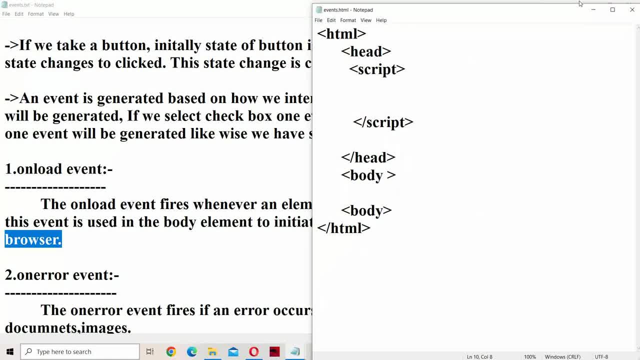 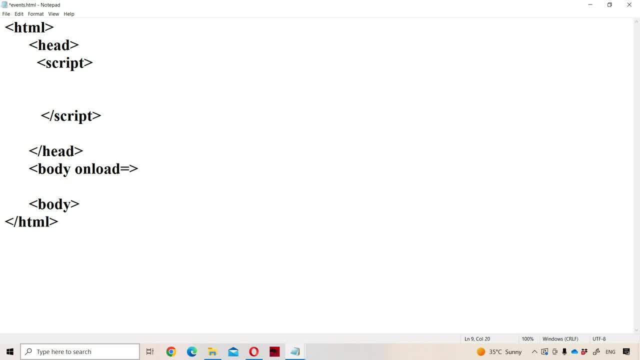 Let us see an example for the onload event. So mainly we use this onload event on body tag, So onload is equal to: let us call a function, Let. name of the function is hello, Hello. Now let us create a function in the script tag, So function. what is the name of the function? Hello, Hello. Let us display an error box here. Error box- Error tau. Error tau, Hello. 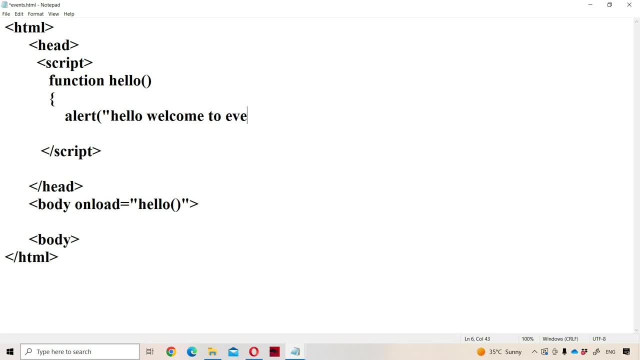 Welcome to welcome to events. Welcome to events. Next to close the function. So whenever this web page is loaded in the browser successfully, then onload event will be filed. Onload event will be executed. Here onload is equal to hello, So here we are calling hello function, So control goes to the hello function definition. So here we have an error box. 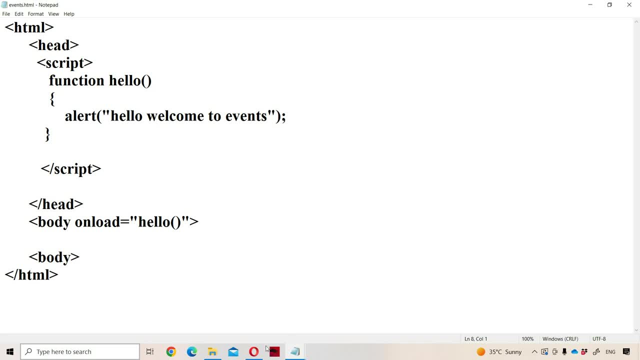 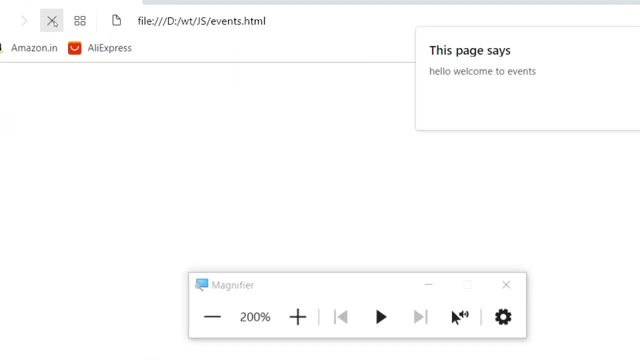 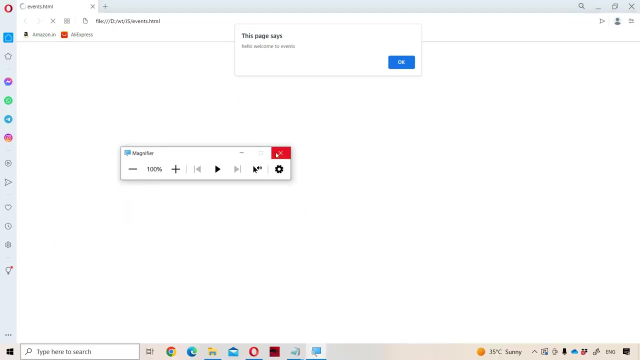 Hello, Welcome to events. So that error box will be printed. So let us see, let us execute now If we see the output here. So whenever we refresh the web page here we got the error box. What does error box contains? Hello Welcome to events. So this is about onload event. So whenever the web page is loaded in the browser successfully, then automatically onload event will be executed. 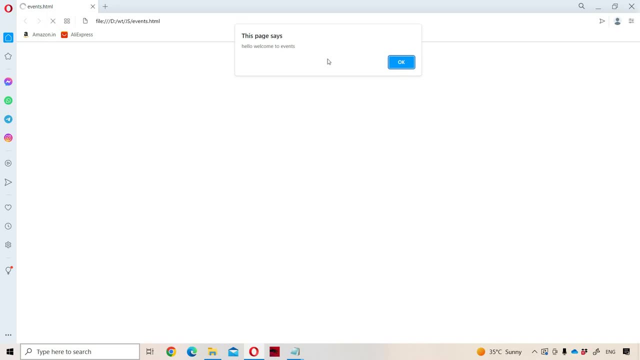 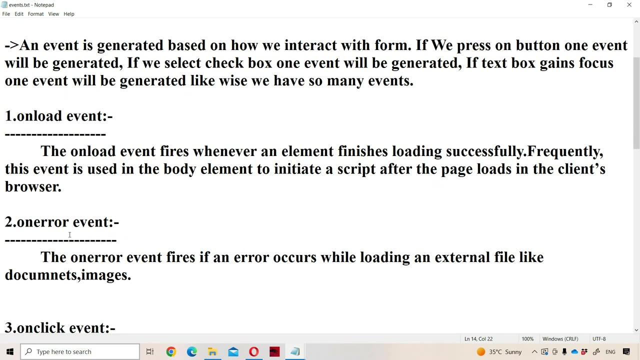 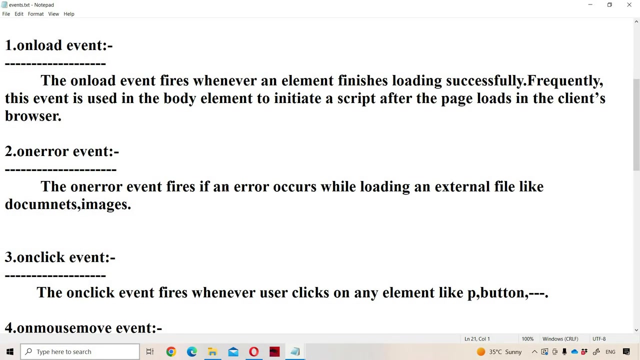 Okay, If we, if we reload the web page, then this alert box will get displayed. Okay, Now let us see the next event, That is on error. Now let us see the second event, That is on error event. On error event files: If an error occurs while loading an external file, like documents and images. So if there is an error while loading a document or image, then onload event will be executed. 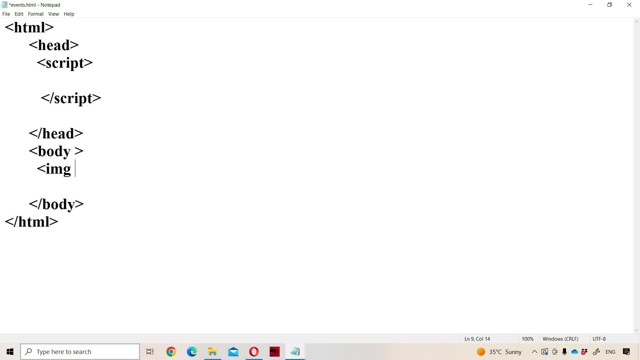 On, error event will occurs. Let us have an image here. I am GSRC, equal to here in my system. in D I have a folder called WT. In WT, a file called JS image is there. Next, let us display with 500 pixels height as well as 500 pixels width. 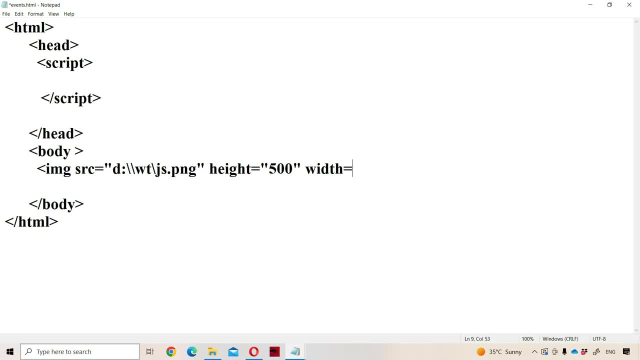 On error event. once they are onloaded, then the image gets displayed, 400 pixels with On error event. next, let us display some alternative text. If the image is not displayed due to any sort of problem, then this text will get displayed. 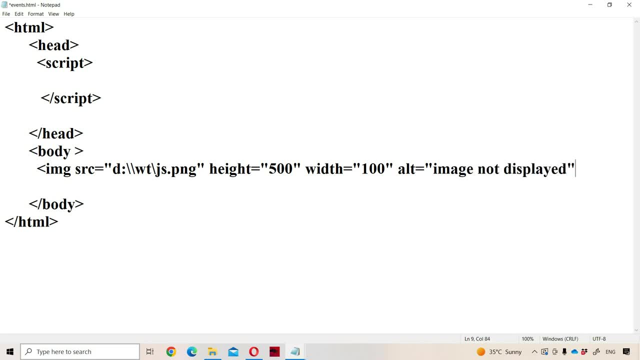 Image not display. OK, No, Let us run the program whether this image is are displaying on, not. Yeah, there is no problem here. we got the image. Now let us go some modifications. yeah, let us do some modifications now. uh, that is. uh, let us change the name of the. 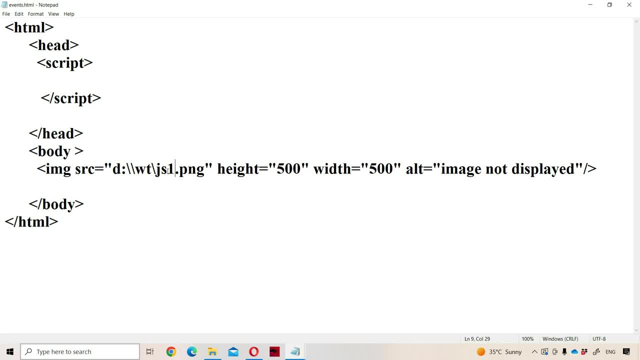 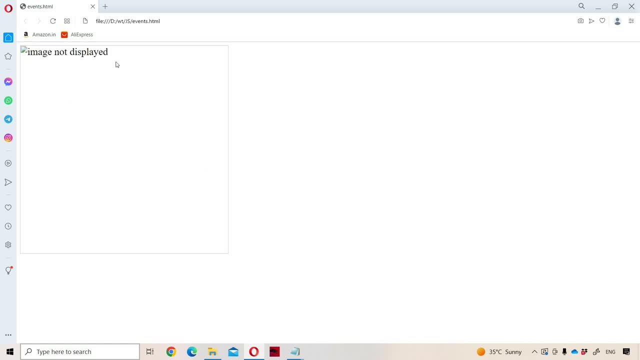 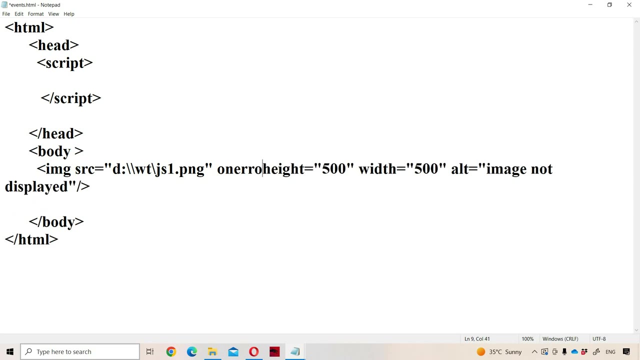 file to js1 with js1 no file. no file is there, so we don't get any output now. so now alternative test: got displayed, image not displayed. okay, uh, now execute on error event. execute on error event so when on error event will gets executed if the image is not displayed. 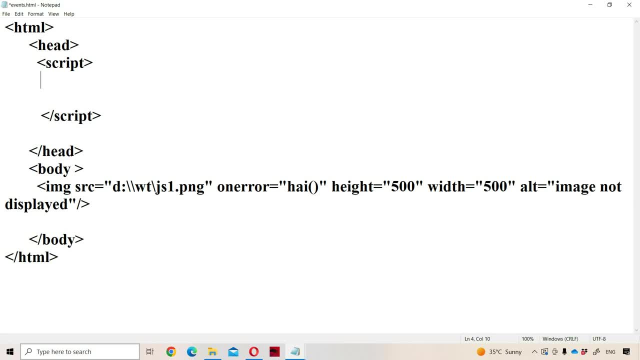 due to any sort of problem, then on error event will gets executed. so let us define a function with the name hi, with the name hi. now let us display some alert box, alert box. so alert of hi, alert of alert of hi, alert of hi. now let us close the function now. let us close the function here with the name js1. 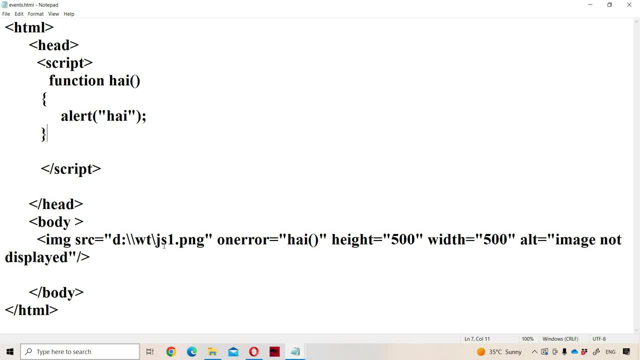 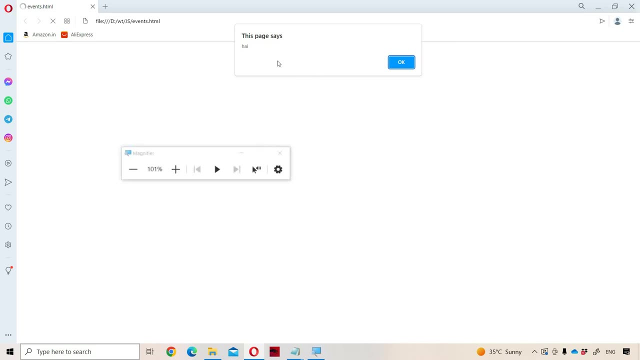 no image is there, so there is a problem of while loading the image. so on error event will gets executed. on error equal to hi, so hi function definition will gets executed. yeah, if you observe here, here we have a alert box with the message hi, with the message hi, okay. 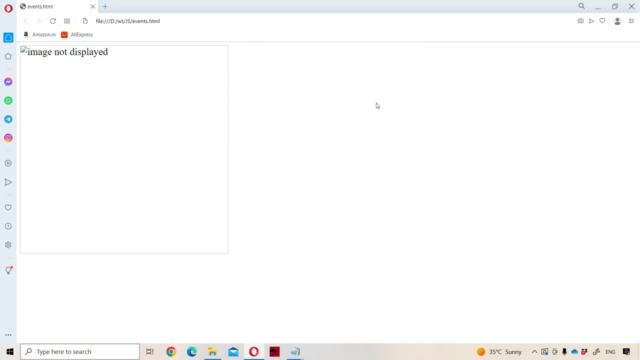 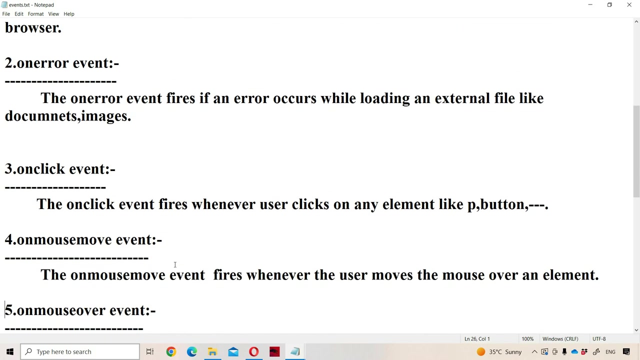 so this is about on error event. okay, so where we need to call the on error event while loading any base or while loading a document, okay, now let us see about the next event, that is, on click event. on click event finds whenever user clicks on any element. it may be any element, so paragraph element or pattern element or 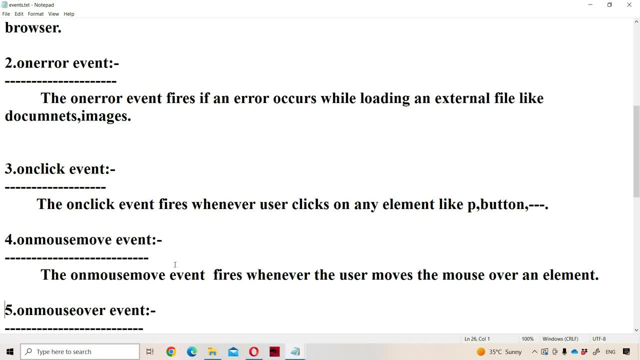 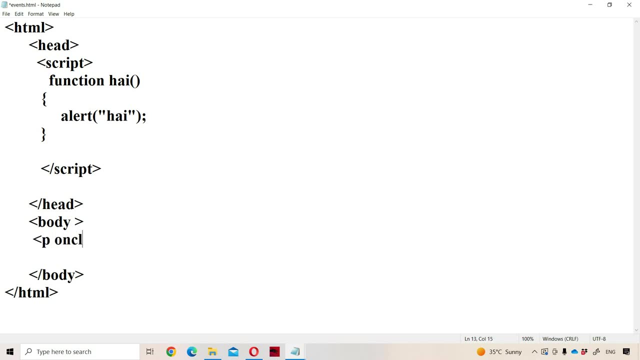 image element or header element or some uh uh bold tag element, italic tag element on any element. if click on a particular element, then on click event will get executed. okay, now, instead of the body tag, let us use the paragraph tag element. so p on click is equal to on click is equal to. let us call. 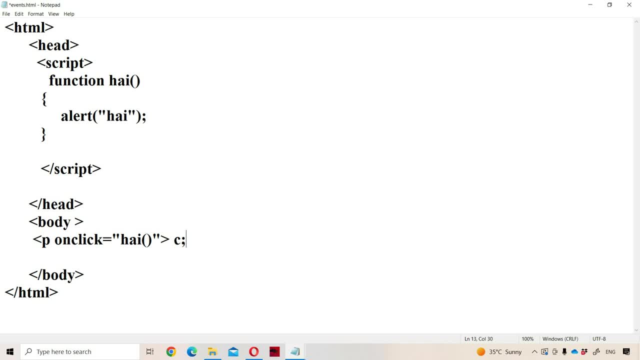 high function. uh, so click on me. so here the test is click on me. so not only paragraph, we can use button or any other control also. there is no problem. okay, now let us run the program. so here we have a click on the paragraph. let us click on this one. so if we click on the paragraph then we 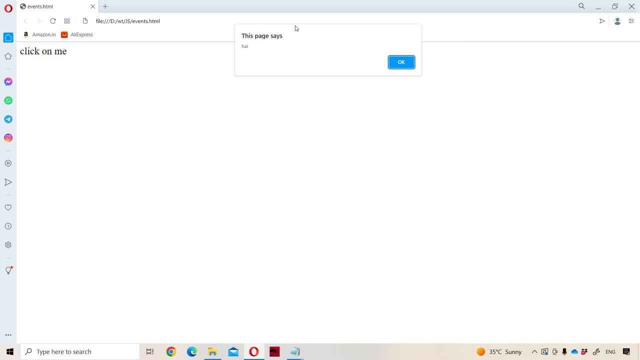 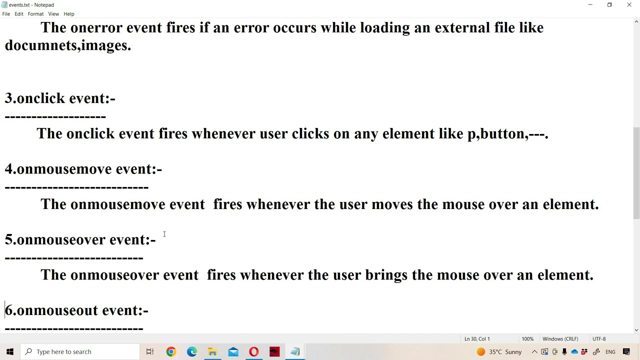 got the element box because of for click event. so whenever we click it on the paragraph, then on click event will gets executed on click is equal to high, so high function definition got executed now. now let us see the next event, that is, most events on mouse move. so on mouse move event will finds: 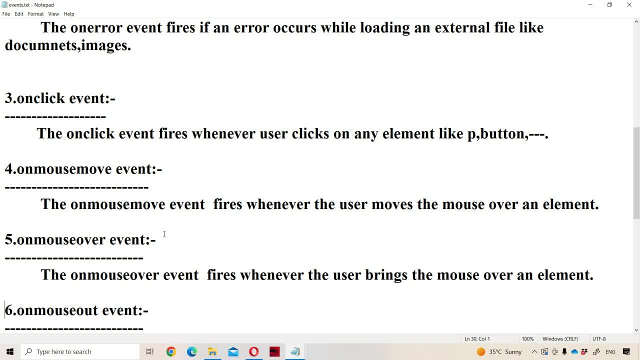 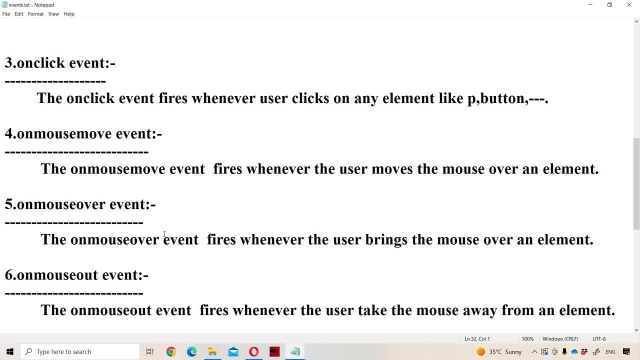 wherever the user moves the mouse over here element. so if we move the mouse over an element, it may be any element: paragraph element or image element or button. uh, it is our choice. next, on mouse over event files: wherever the user brings the mouse over here element. so when we, when we places the mouse, 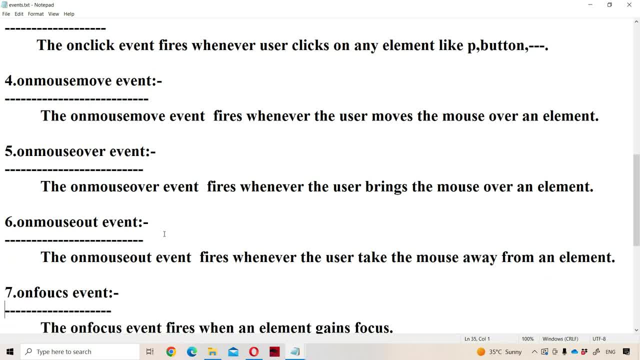 over an element, then on mouse over element will gets executed. next, on mouse out event files whenever the user takes the mouse away from the element. so here we have three mouse events: on mouse move event files whenever we you remove the mouse on your element. uh, where he has almost over. 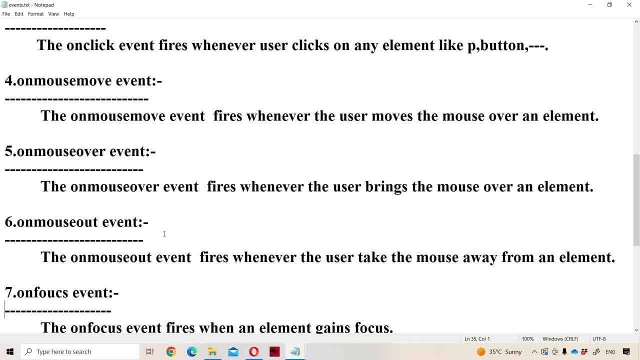 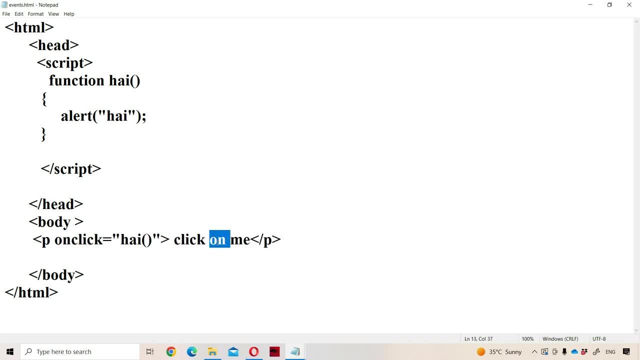 files whenever the user breaks the mouse over your element on mouse out, even fights whenever the user take the mouse away from the element. okay, so we have uh three mouse events, so let us execute uh those events uh by by taking any base. why? because here image means uh we have uh bigger canvas, so img src equal. 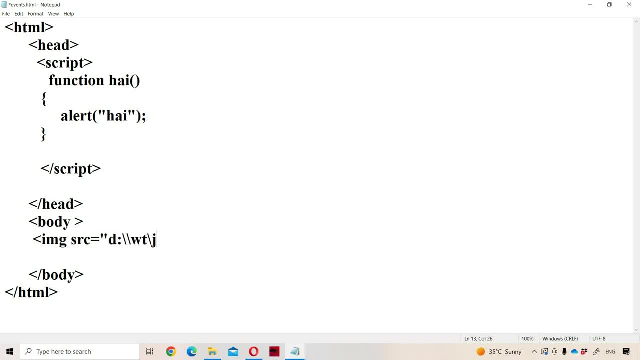 to so. d colon, wt folder. name of the file is jspng, jspng, uh. height is uh. height is uh. let the height is 500 and next to let the width is also 500, 500. so on, mouse on mouse, move equal to. let us execute high function. let us call high function. 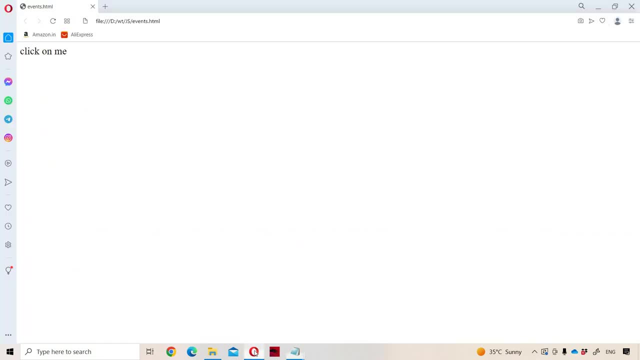 on most move. okay, ctrl s, let us run the program. let us run the program. yeah, if we move the, if he places the, if we move the mouse, if we move the mouse over the image, then what will happen on mouse move will it gets executed, so on mouse move equal to high. so the talent box got printed, okay. 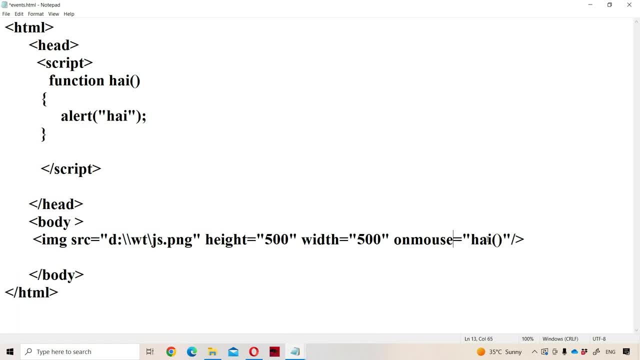 now, in place of on mouse move, let us place on mouse over, on mouse over. next, let us have one more function, uh, one more event. on mouse out equal to, on mouse out equal to let. name of the function is hello, hello, so let us have one more function. 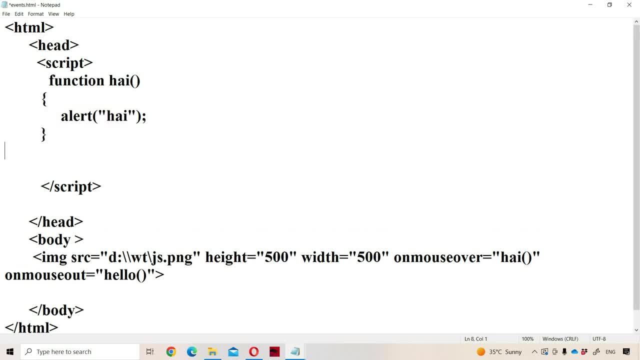 let us have one more function: ctrl c. that name of the function is hello. so when hello will get executed when the mouse cursor is placed away from the element. if we move the mouse cursor away from the element, then on mouse out even will gets fired. let us run the application now. let us 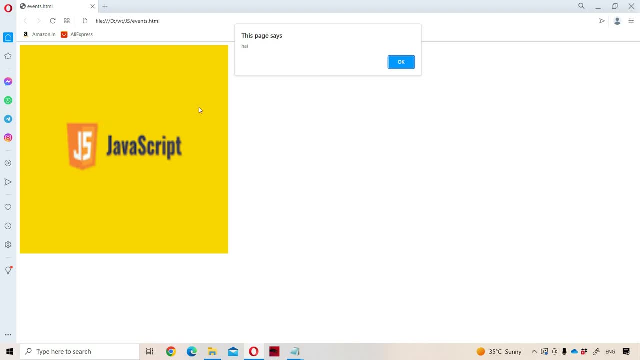 run the application. yeah, if we move, if he places the mouse over here, the limit then almost over event will gets executed and high function got executed next. next on mouse. we have on mouse over also in order to execute the todd. mose over on mouse out and let us remove this function. 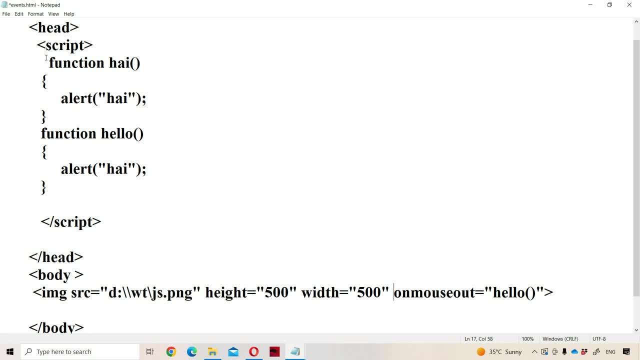 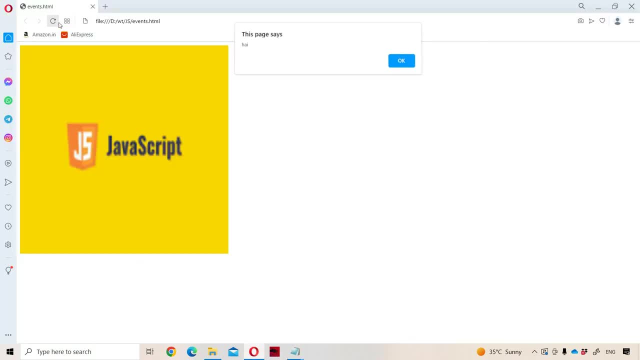 let us remove this function on mousse out. so what is our most out function definition? hello, hello. let us run the program now. yeah, yeah. and now. if the boss cursor is warrior element, then the lower box got printed where he has if he move the mouse away from thek. 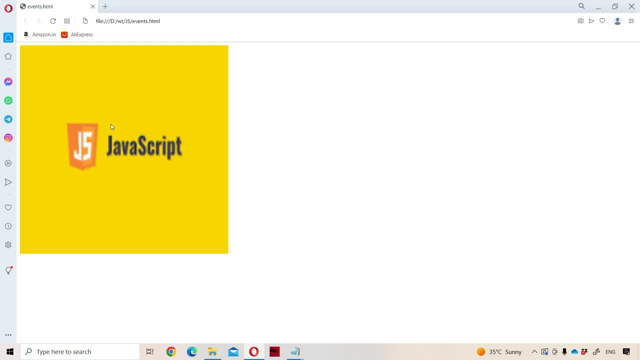 9. now if the mouse cursor is over your element, then no error box got printed where he has. if you move the mouse away from the default criticisms, now all right, so let us run his operation here. yeahp, didi Program is over, so it getsakan. that's all right right now, and if you move the mouse over, hit Ты. 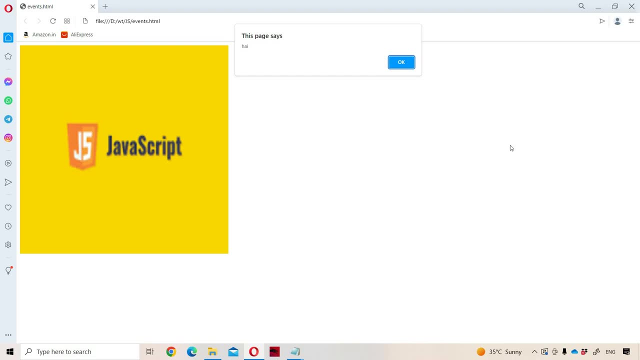 away from the element, then on mouse forward will get executed. I am sorry, on mouse out will get executed, so when on mouse out event will get find when we move the mouse cursor away from the element, then on mouse out will get executed and the alert box got printed. alert box contains: 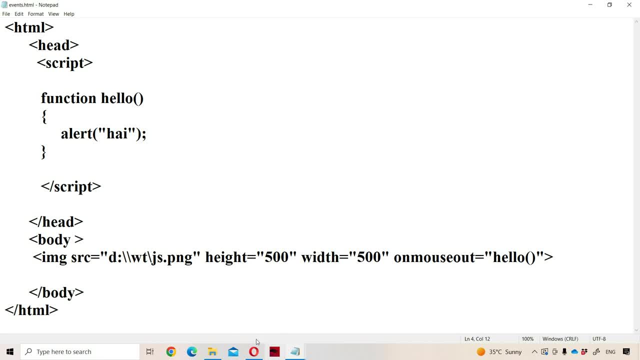 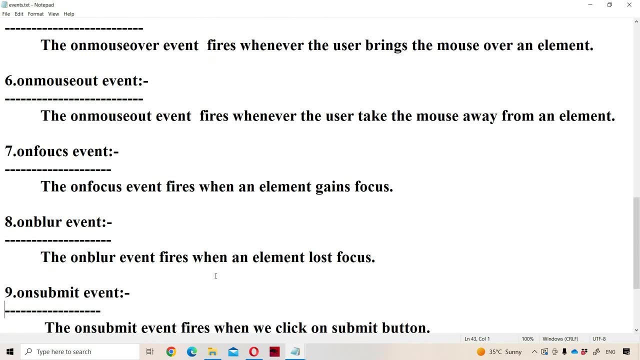 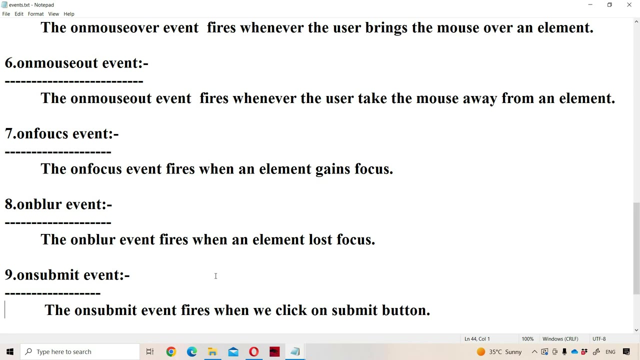 some high message. so here, what is the alert box? high message. now let us see the remaining controls. next one is on focus event, on blur event. on focus event finds when an element gains the focus, whereas on blur event finds when an element lost the focus. so mainly. 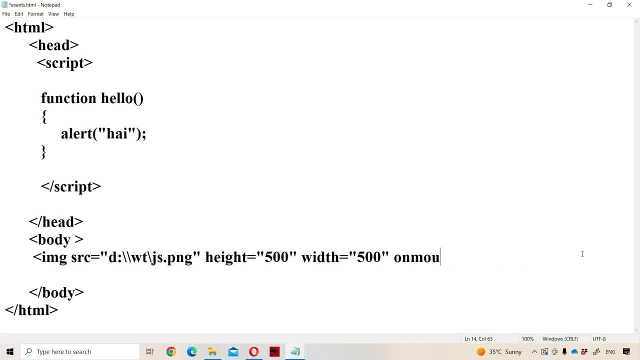 we uses on focus and on blur while working with text boxes. so let us create the text box now. input type equal to text. input type equal to text. next, on focus equals to text. input type is equal to hello. so whenever we places the cursor in the text box, then 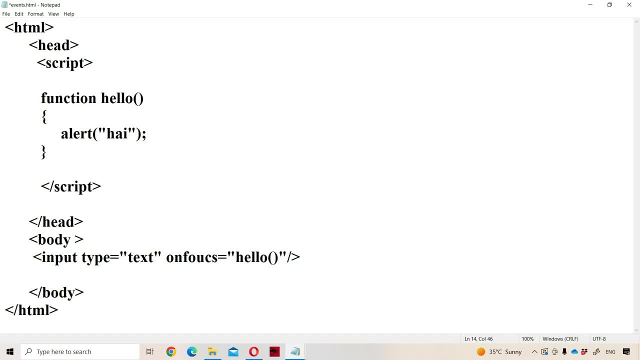 what will happen whenever we places the cursor in the text box then on focus event will get find on focus equal to hello. so hello function definition, that is, the alert box will get printed. so let us see the program. so whenever we places the cursor in the text, 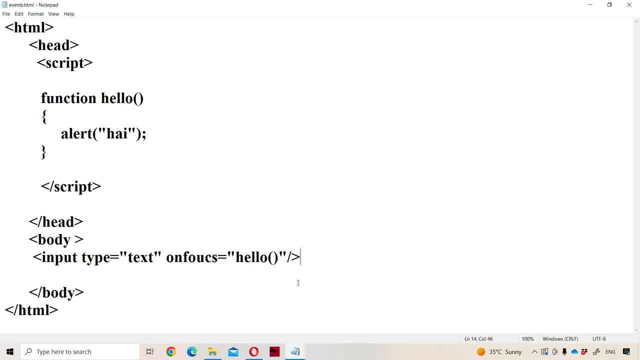 box. then what will happen? yeah, so let us see the program. some error is there. on focus equal to. on input type equal to text. on focus equal to hello. yeah, there is no mistake. next function: hello, function hello. let us see where is the error. input type equal to. 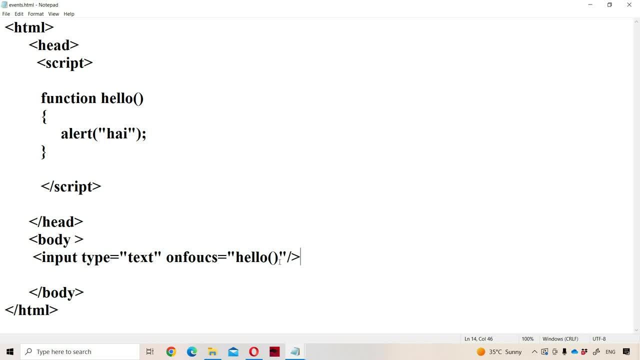 text on focus on focus equal to hello. yeah, hello, no problem is there? so input tag is closed, as well as body tag is closed in the script section. so function, hello. let us save the program one more time. Yeah, now let us run the program. yeah, some error is there. so here, what is the element? 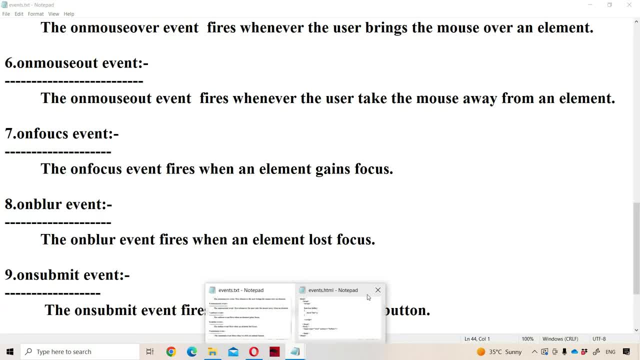 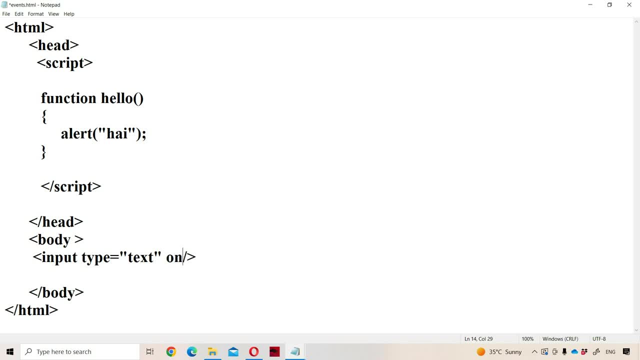 here. what is the event on focus and on blur event? yeah, yeah, yeah, let us let us input type equal to text. let us type one more time: on focus, equal to on focus, equal to let. name of the function is hi on focus, equal to hi, so function. 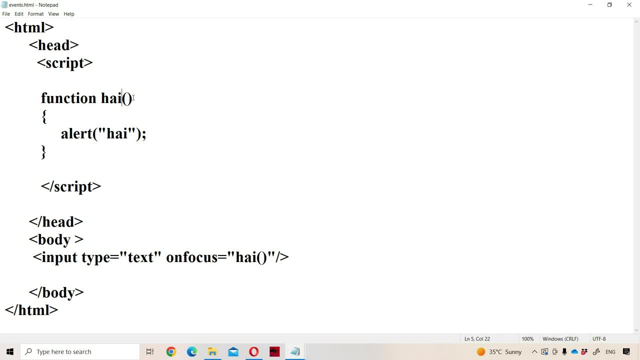 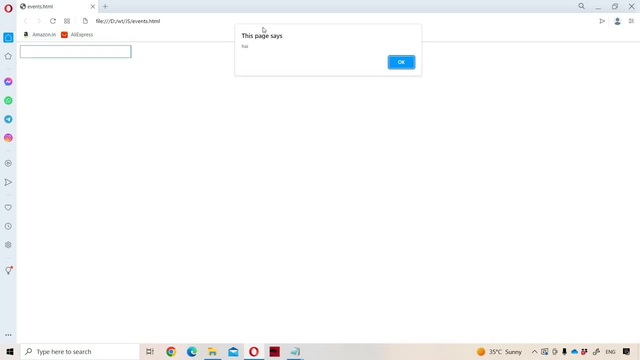 function hi, function hi, yeah. now let us see the output. yeah, whenever the text box gains the focus, whenever the text box gain the focus, whenever we places the cursor in the text box, then on focus event will gets executed, then that automatically, that alert. 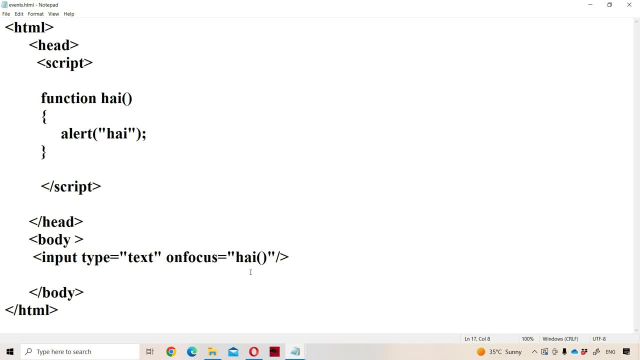 box got printed. Now let us see about: on blur event on blur. So this is the on blur event on focus. let us write blur. so when on blur event will gets executed whenever an element leaves the focus. that means whenever, whenever we have taken 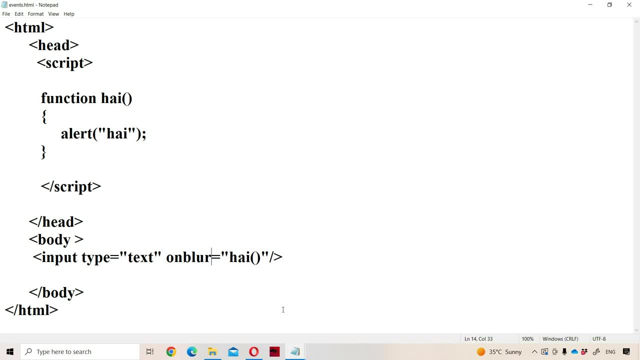 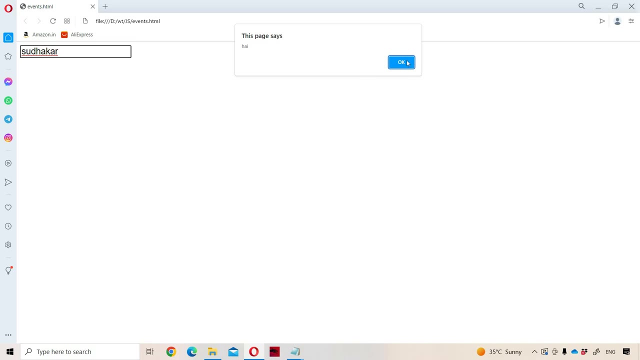 the cursor away from the text box, then, on blur, event will gets executed. okay, Let us see the output here. yeah, let us type some data in the text box, Sudhakar. so whenever we move this cursor away from the text box. okay, then on blur, event will gets executed. 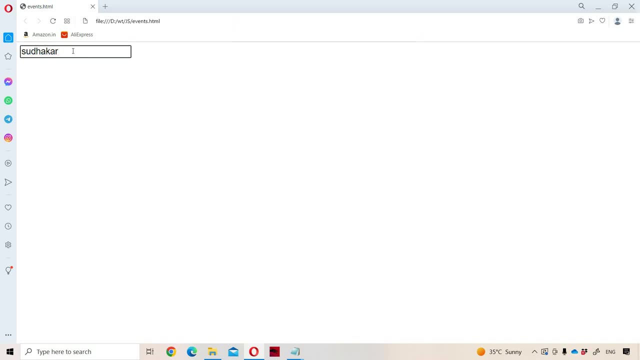 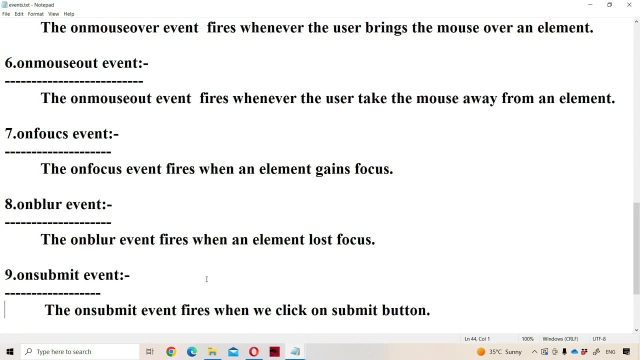 okay, Yeah, now the cursor is in the text box, so whenever we have taken the cursor away from the text box, then on blur event will gets executed. Now let us see two more events on submit and on reset event. on submit event files. 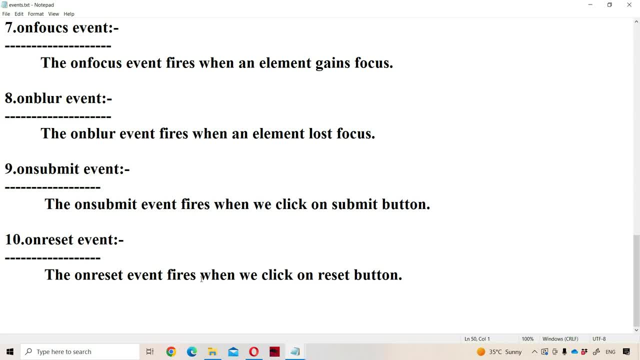 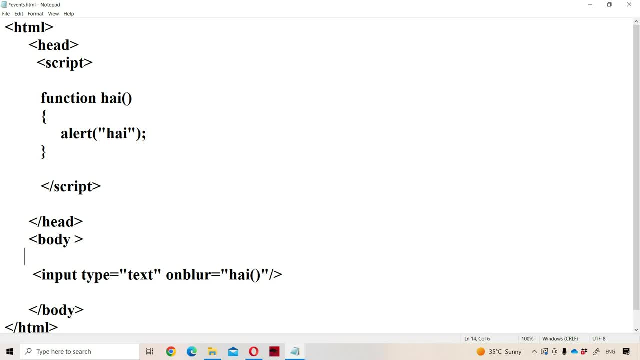 whenever we click on the submit button, whereas on reset event files whenever we click on the reset button. So here now we have to create a form. let us have a form. so form form on submit. on submit event. 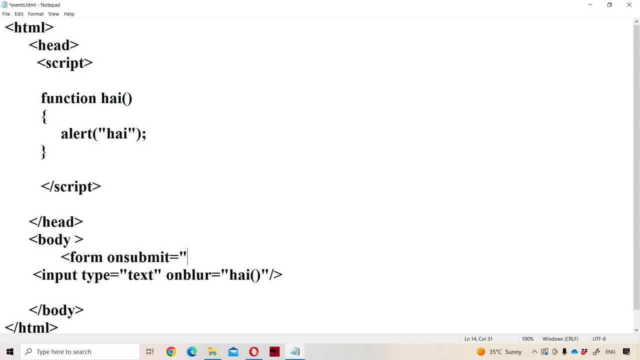 Okay, On submit equal to. on submit equal to hello, hello. next, on reset equal to hi. now we need to define two functions. yeah, we need to create two buttons. the first button is what submit button. so input input type equal to submit. input type equal to submit. next, 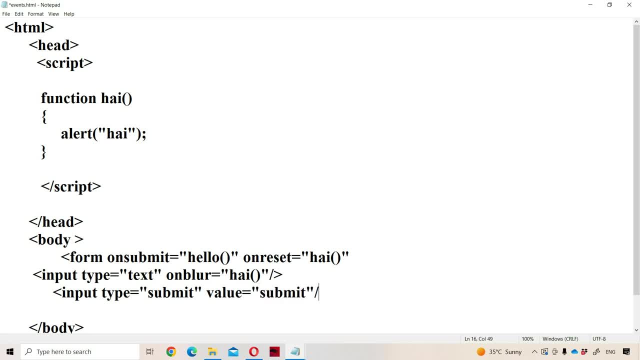 value is equal to submit. So if we click on this submit button, then on submit event will gets executed. so hello alert box will gets displayed. Next, if we click on this reset button: input type equal to. input type equal to reset. 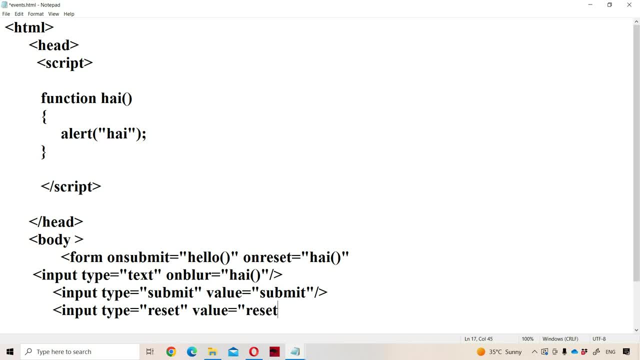 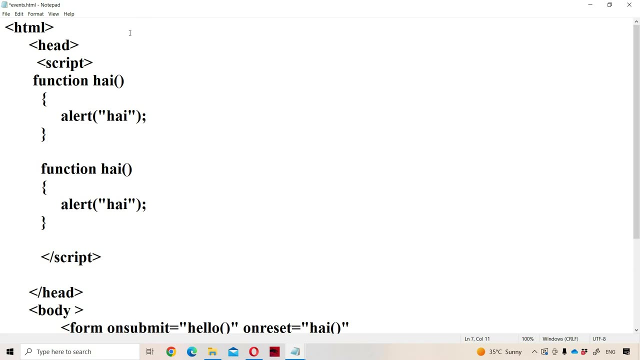 value equal to reset. If we click on this reset button, then on reset button, on reset event will gets executed. Now We need to define one more function: control c. so what is that? function hello, Let us define hello function. hello function. so function hello. let us modify the function. 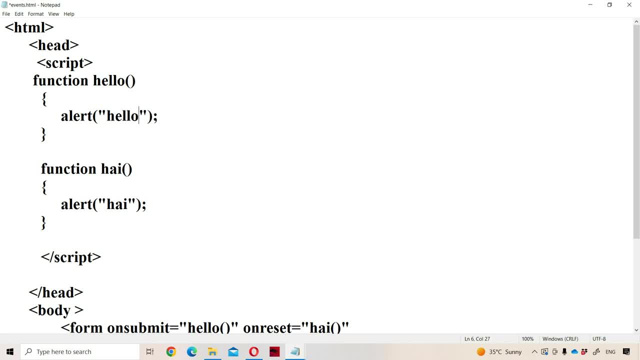 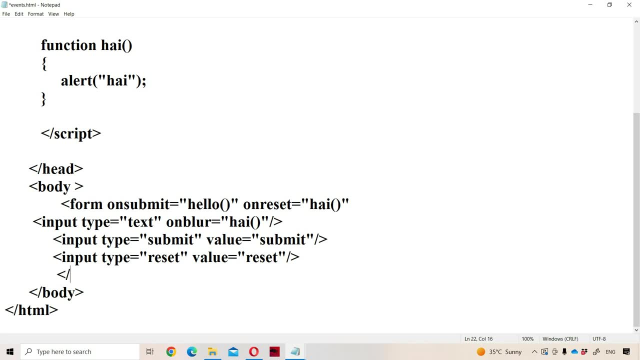 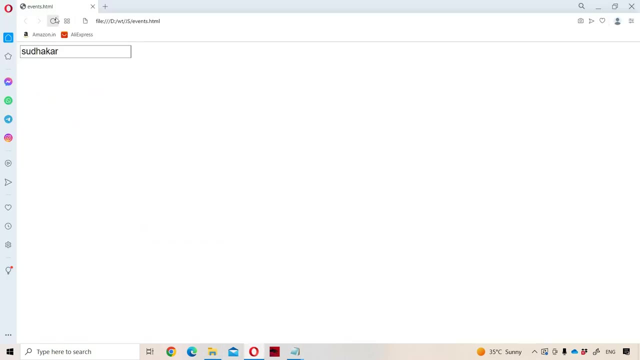 definition to hello. So if we click on the submit button, then what will happen? hello function definition will gets executed. if we click on the reset button, then hi function definition will gets executed. Now Let us run the program. yeah, let us run the program. let us click on the submit button. 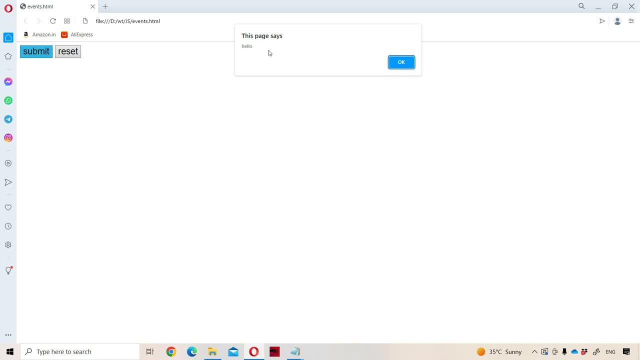 so whenever we click on the submit button, then on submit event will gets executed on submit equal to hello. so hello function definition. hello alert box got printed okay. hello alert box got displayed okay, if you see here, hello, okay. next let us click on the reset.